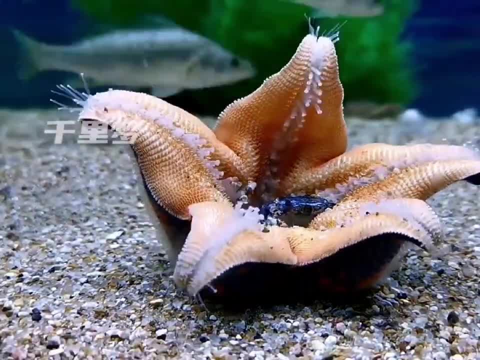 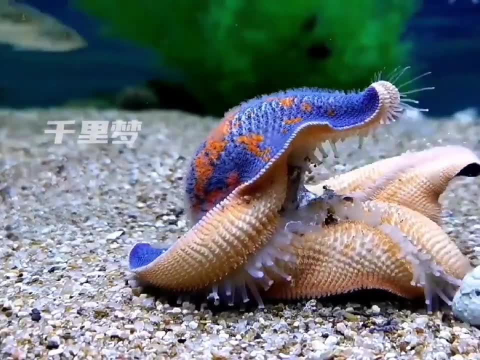 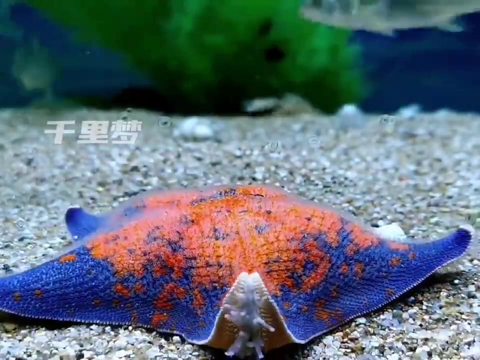 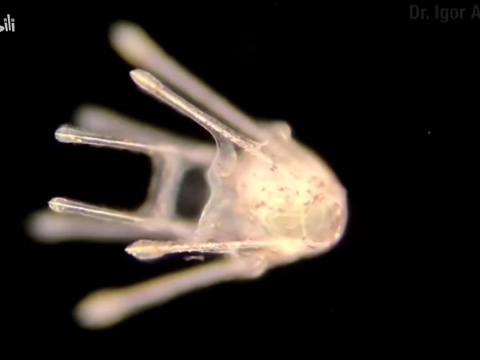 Now tell me, are you impressed or not? If you're not, don't worry. Starfish will always be able to satisfy your curiosity. For example, their unique growth and development pattern is absolutely unparalleled in the animal kingdom. First, let's take a look at this little guy, the larva of a starfish. 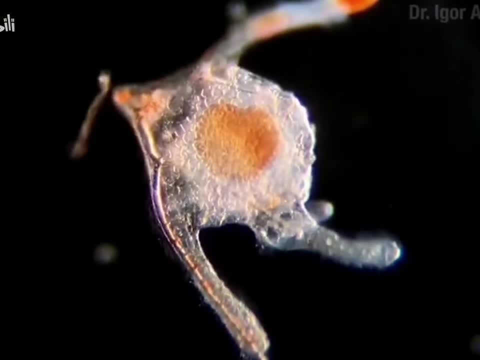 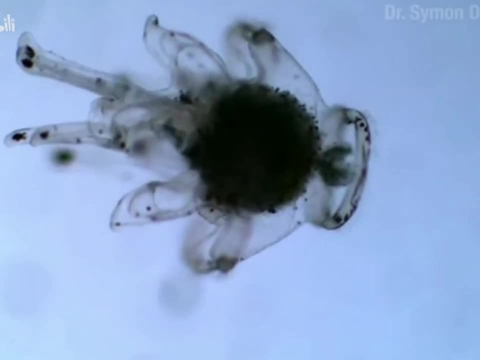 It looks nothing like an adult starfish, but that's not too surprising, as there are many similar examples in nature. However, when this larva reaches a certain stage, it not only grows numerous tentacles, but it also grows a lot of other things, For example: 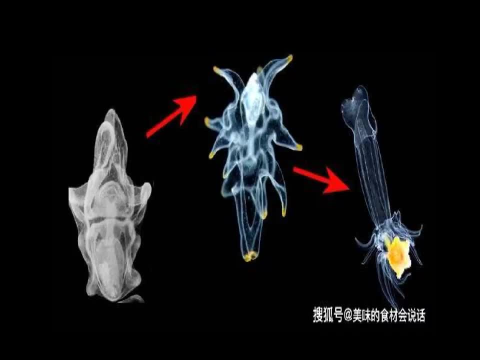 it has numerous tentacles, but also develops a five-pointed star-like structure on one side of its body. Eventually, the starfish larva settles to the ocean floor and the five-pointed star detaches. That's right. this five-pointed star is the actual adult starfish. 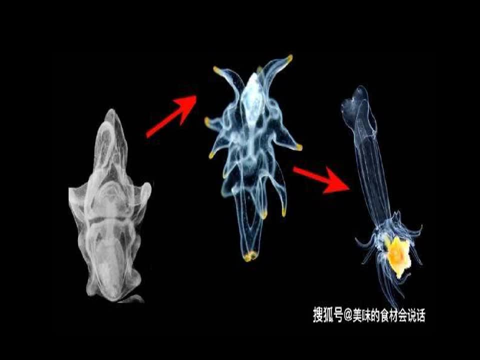 In other words for starfish, it's not that the younger version of you grows into the adult version of you, but rather the adult version of you grows into the adult version of you. That's so cool that it's practically friendless In our era. there are four other types of. 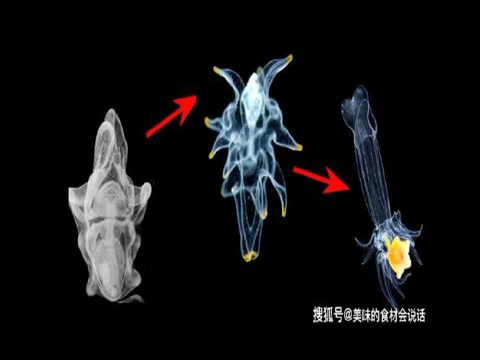 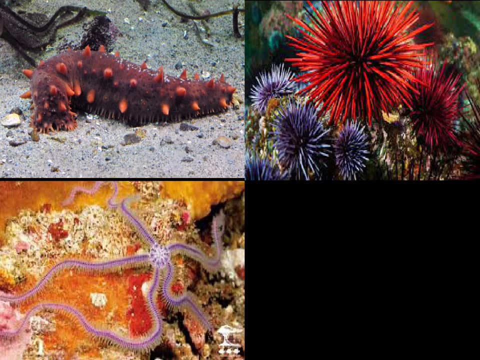 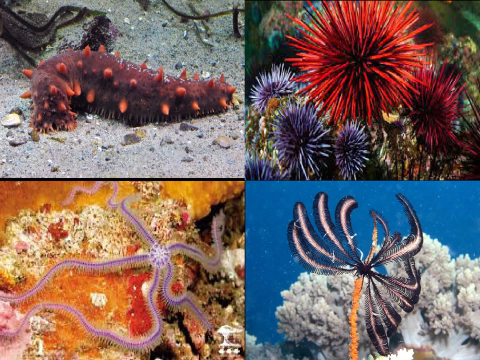 animals that also belong to the echinoderm group. along with starfish, These are sea cucumbers, sea urchins, brittle stars and crinodes. In short, if you see an animal with a name that starts with C, followed by a word that has nothing to do with the ocean, there's. 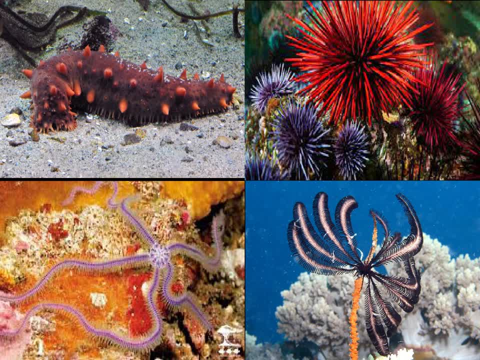 a good chance, it's a starfish. We know that scientists classify certain animals into a large group because they share some common features. However, this commonality among echinoderms is not apparent in their outward appearances. Starfish look like stars. sea urchins are spiky bowls, sea cucumbers. 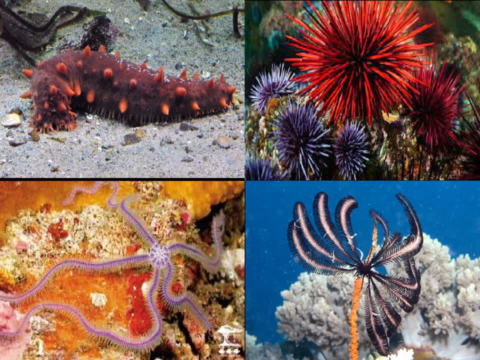 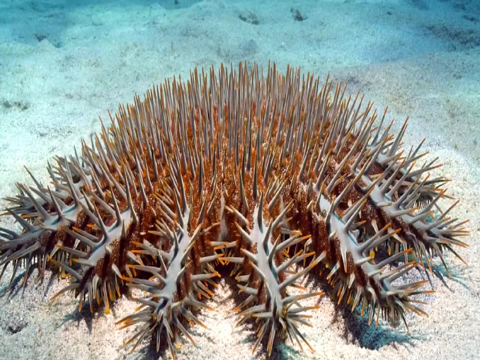 are called sea cucumbers by foreigners because they look like pickles, crinodes resemble flowers And as for brittle stars, they look like severely underdeveloped starfish. Alright, forget what I said. Yes, starfish might not necessarily look like stars, and sure sea urchins can also take on a coin-like. 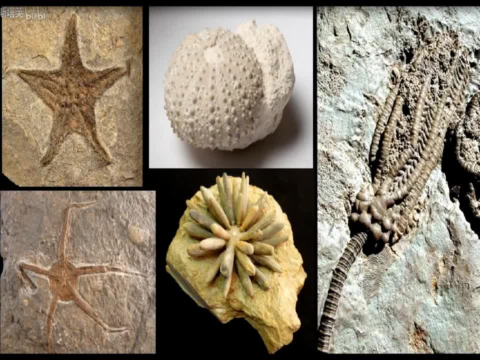 shape. Fine. the point is, the appearances of echinoderms are incredibly diverse and unpredictable. I've always wondered if animals like starfish and sea urchins had gone to the same place. What would today's paleontologists make of the vast array of star-shaped and spiky-ball? 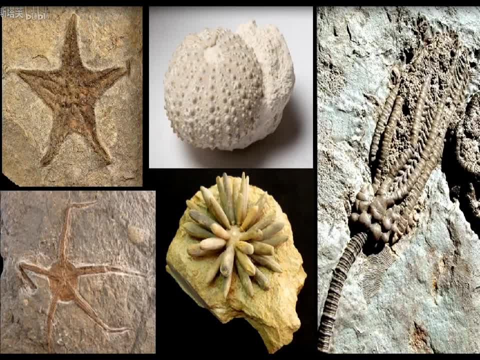 fossils. It's hard to imagine the bizarre and monstrous creatures they might reconstruct from such evidence. Speaking of bizarre and monstrous creatures, I'm reminded of the ancient echinoderms that looked like a parade of ghosts and goblins. Let me give you a few examples to help you. 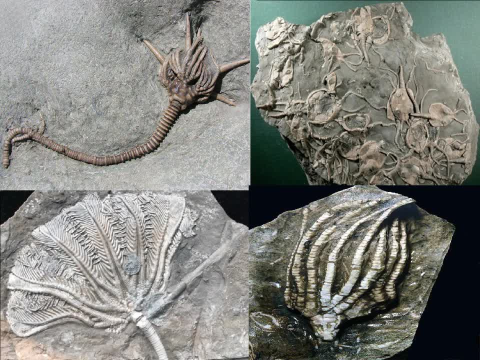 get a feel for them. If we think of evolution as a process of natural selection where only the fittest survive, it's hard to say what kind of intelligence contest the echinoderms were engaged in. Generally, early echinoderm ancestors evolved into a sessile, filter-feeding lifestyle on. 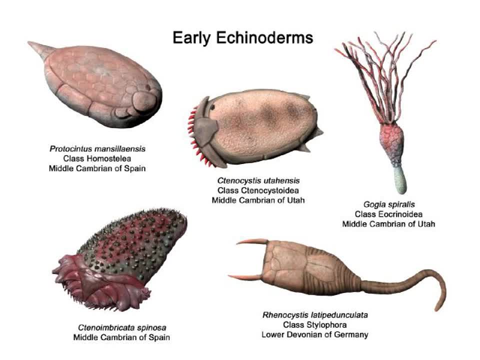 the ocean floor. While this may not seem particularly unusual, the sedentary filter-feeding lifestyle is typically stable. But what about the echinoderms? Well, the echinoderms are very simple And the body structures required for it don't need to be overly complex. 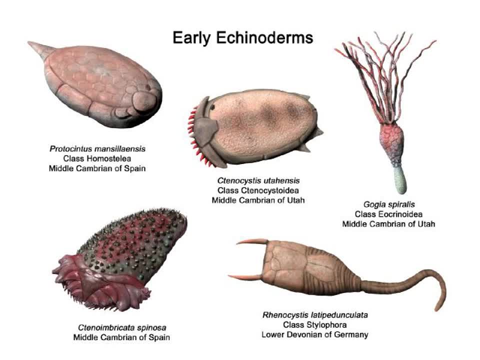 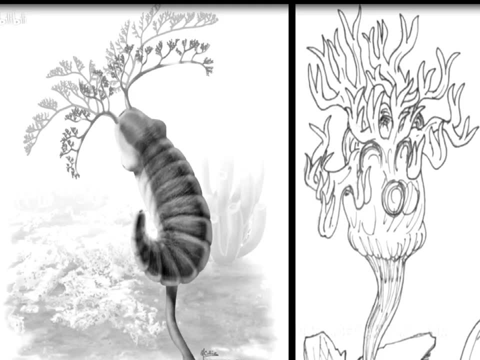 So, evolutionarily speaking, these creatures should appear relatively conservative. However, echinoderms are not ordinary animals. Their earliest ancestors might be traced back to creatures like this, Although their shapes are somewhat peculiar. their appearance is strange. The echinoderms are not ordinary animals. 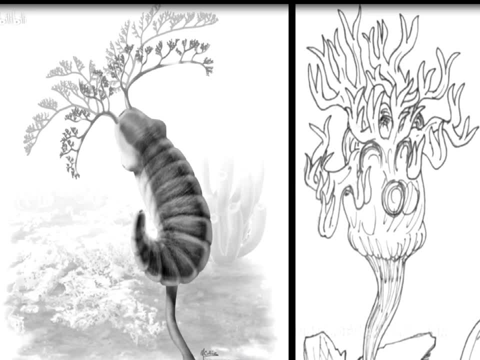 There's no way to define the appearance of the echinoderms. They have an unusual, unique shape. Their appearance is still somewhat acceptable. It's easy to tell which end is the mouth and which is the anus. Their bodies display bilateral symmetry. 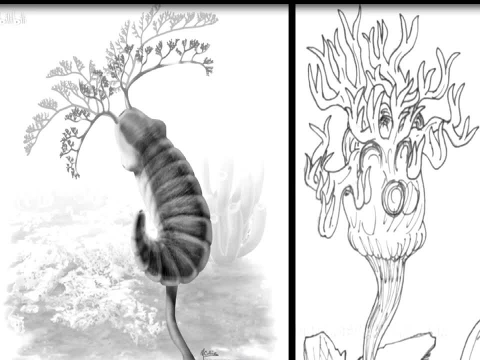 And while the unique little tail might seem out of place, it's still a meaningful structure. But then the echinoderm's evolutionary course took an unexpected turn. Usually, when organs and structures are lost during an animal's evolution, they don't really. 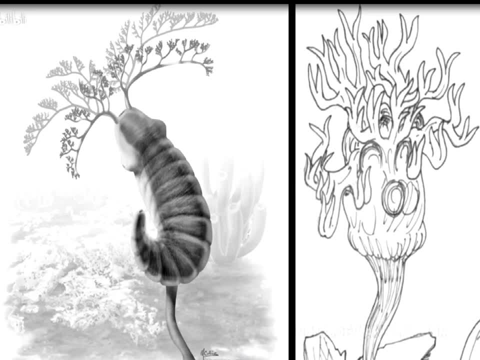 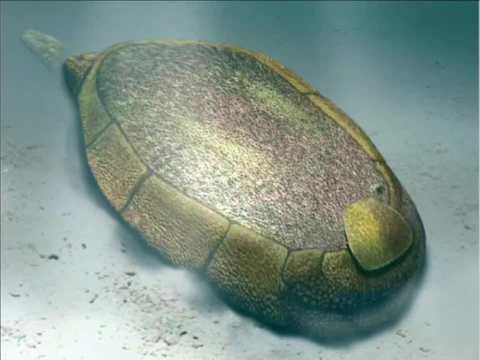 they don't reappear. But echinoderms didn't care about these rules. For example, they first lost the little tail and tentacles around the mouth, turning into something resembling a hot water bottle lying on the ocean floor. Then suddenly they stood upright and the tentacles around the 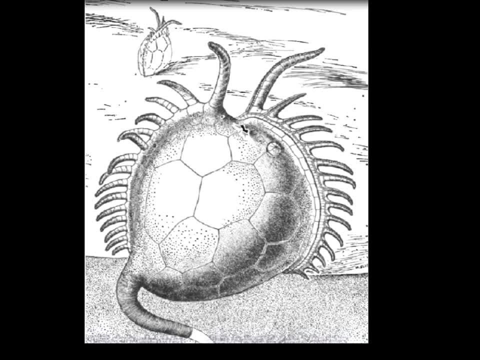 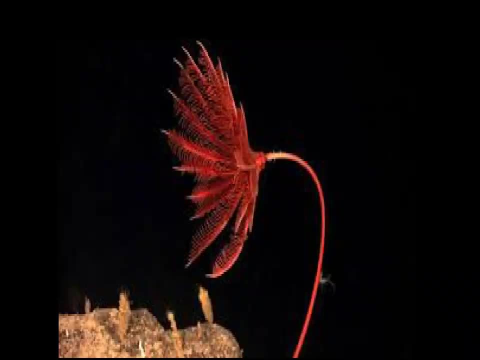 mouth somehow re-evolved. Afterward, one of these tentacles extended into the ocean floor and the tail returned. What kind of bizarre maneuver was this? Finally, this group of echinoderms gradually abandoned their original bilateral body shape, giving birth to crinoids. 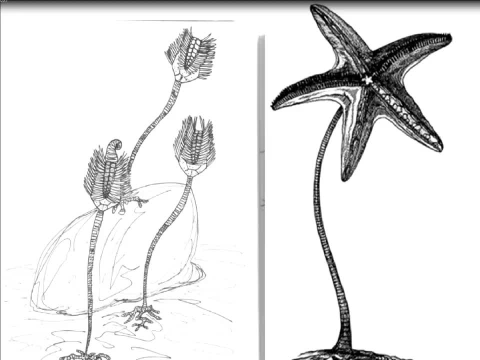 In addition to crinoids, there were several other echinoderms, such as blastodes, which also followed the path of fixed filter-feeding evolution. Although they experienced different body transfers, they were still able to survive. They eventually developed into small flower-like forms Between 200 million and over 400 million. 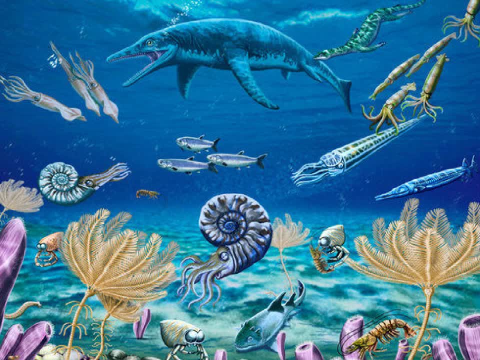 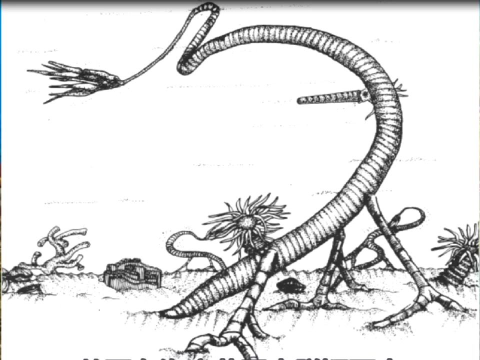 years ago, the oceans were filled with crinoids and blastodes, creating a vibrant and colorful underwater garden full of diverse and bizarre echinoderms. Some crinoids were straightforward in their approach to growth, aiming to become taller, larger and sturdier to stay in the 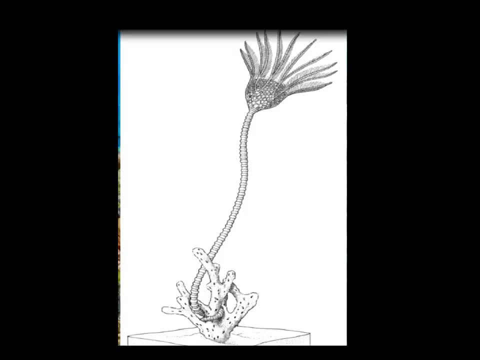 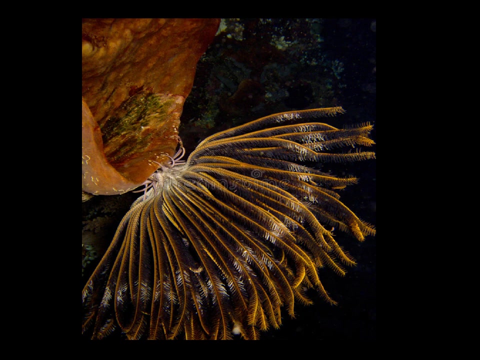 water. Others adopted a more adventurous approach, no longer anchoring themselves to the seafloor but instead turning into vine-like structures, wrapping themselves around other objects and easily relocating whenever necessary. Some crinoids were even more adaptable, attaching themselves to floating objects on the ocean surface, gaining a higher vantage point and 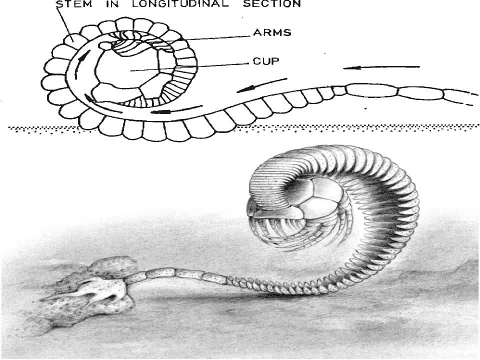 outcompeting other crinoids. Others went as far as becoming predators, capturing small fish and crustaceans attached by hand and engulfing them like a sushi roll. Although these flamboyant and complex prehistoric crinoids have gone extinct, the crinoids that 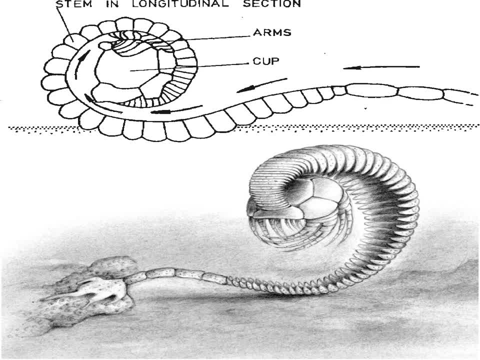 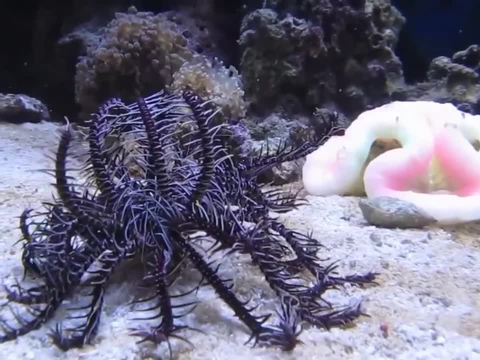 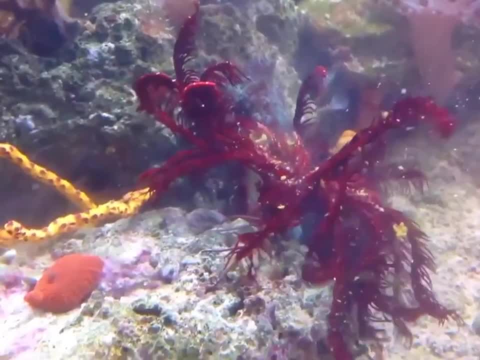 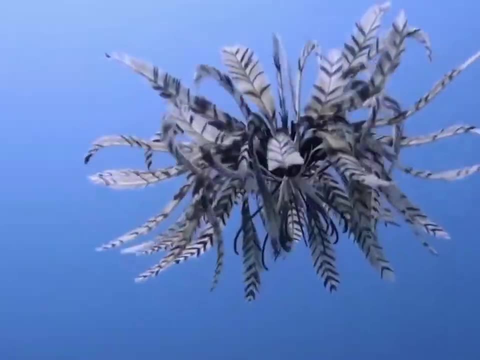 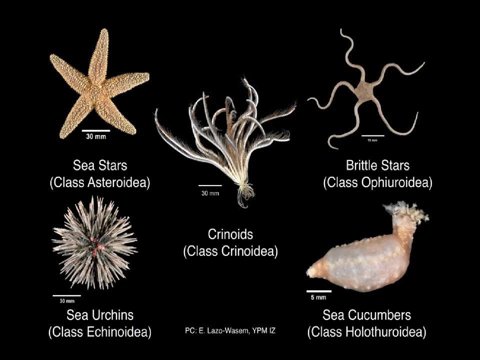 like roots that they can use to walk across the seabed, And some had even evolved into feather stars, which can swim. However, among echinoderms, these creatures that seem to come from another world are just the tip of the iceberg. There is another group of echinoderms that chose to 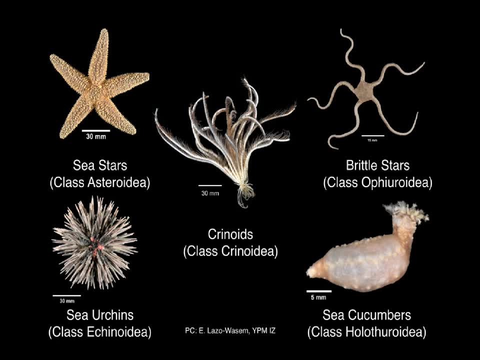 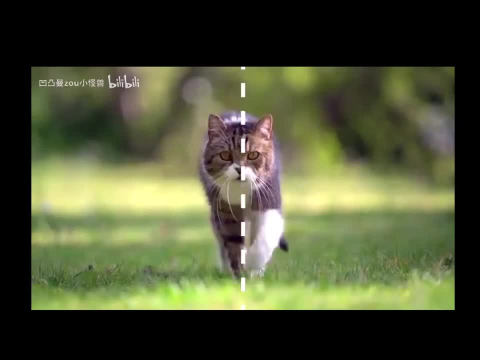 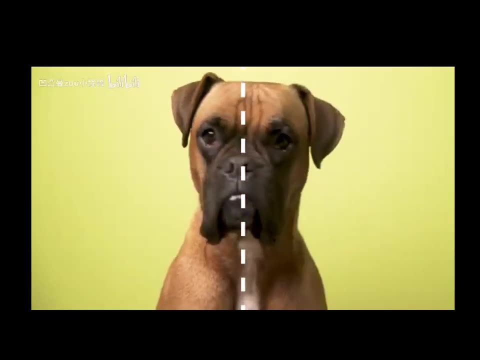 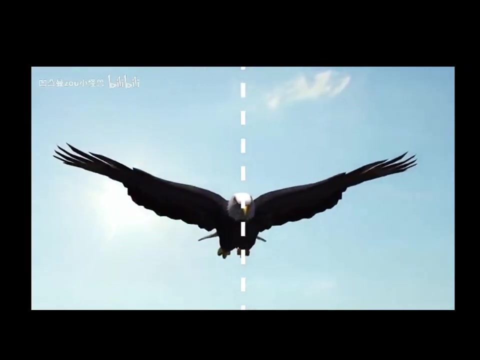 abandon their fixed lifestyle from the beginning and start moving around. generally speaking, When an animal evolves to a free-moving lifestyle, it strengthens its body symmetry, grows legs and eyes and develops muscles and nerves, among other things, But echinoderms don't follow these steps. The first step for echinoderms is to twist their 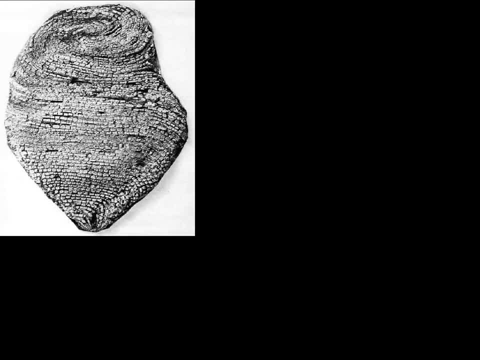 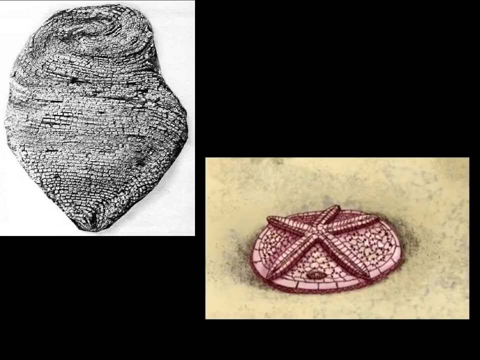 bodies like a hornet. This animal in the picture is called a hornet, It's called a helicoplochoid and it's unbelievable. It twists its body several times, but does it grow legs after that? No, The second step for echinoderms is to flatten themselves. 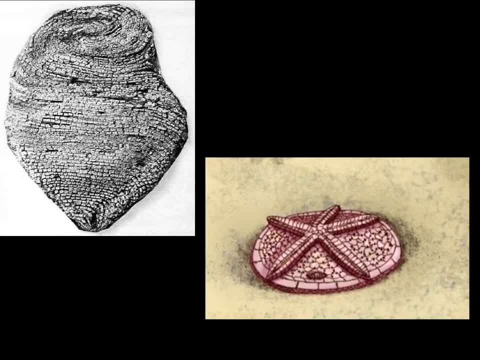 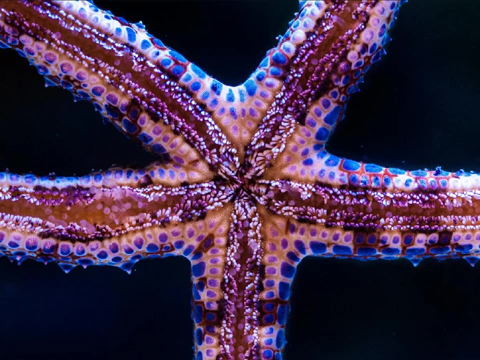 Okay, let's flatten them, but then do they grow legs and muscles? No, The next step is to turn themselves upside down and use the small tendrils it once used to filter seawater to. That's how seastars evolved. It's like humans degrading their hands and feet. 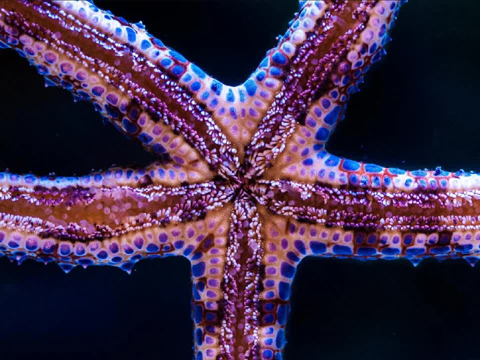 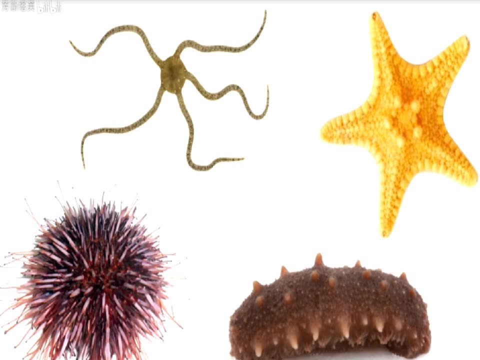 and then standing upside down and moving with their tongues. It's an evolutionary path that's hard to grasp, but that's how echinoderms evolved. But that's how echinoderms evolved, with an evolutionary path that's hard to understand. 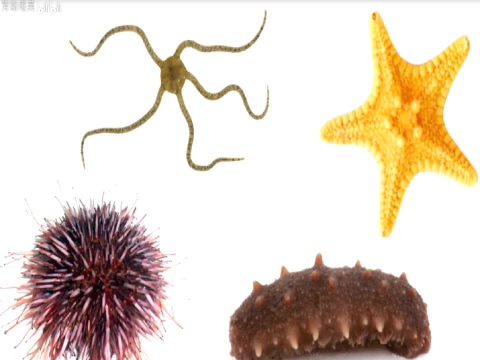 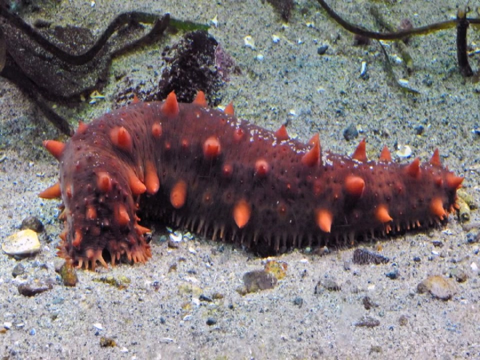 Despite this, they managed to create the most successful echinoderms branch of echinoderms that still exists today, including sea stars, sea urchins, sea cucumbers and brittle stars. Among them, sea cucumbers are perhaps the most difficult to explain. 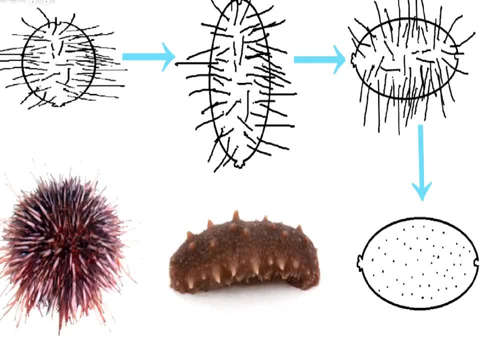 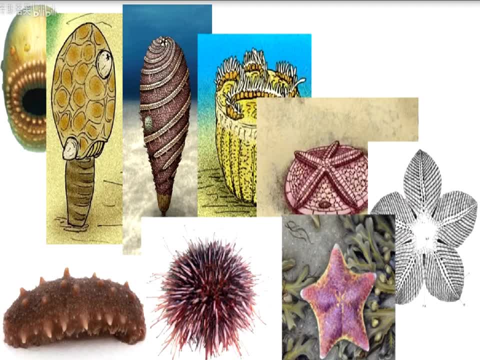 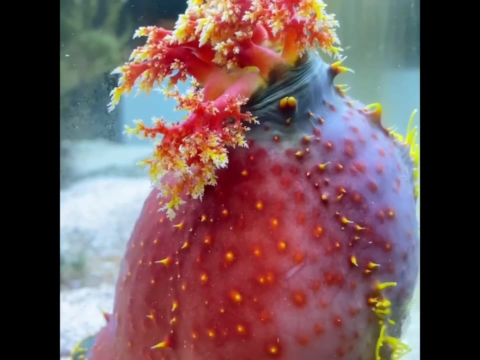 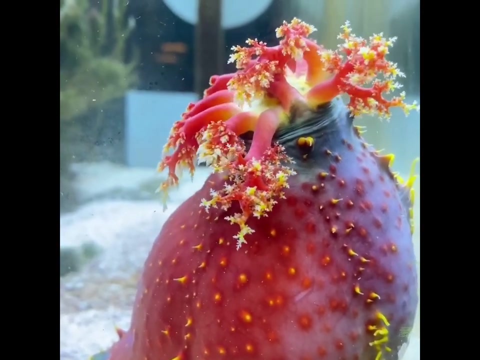 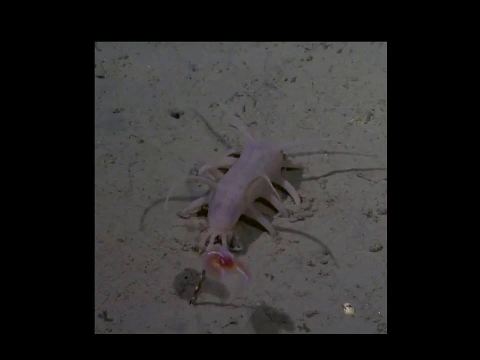 What did BERD do? What did BERD do? What did BERD do? types of sea cucumbers: one could have a truly lavish feast. If you think that sea cucumbers are the bizarre pinnacle of Echinoderm evolution, then you are mistaken. In my opinion, the most 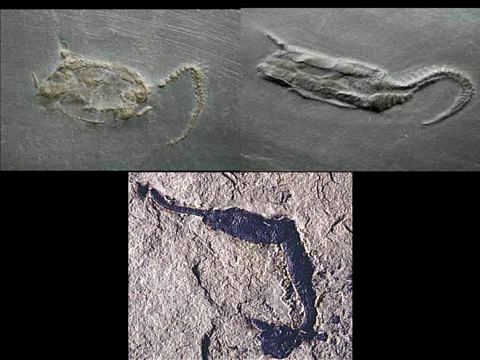 wild and non-conventional Echinoderm in terms of form is not the sea cucumber or crinoid, but the homozoans also known as the Edrioasteros. These creatures are a type of Echinoderm that 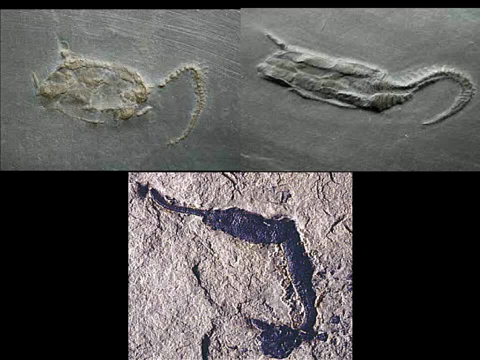 seems to want to be a quiet filter feeder, yet is unwilling to completely give up its mobility. Unlike the Helica playcodes, sea urchins and sea cucumbers, whose bodies still follow some form of symmetry, the homozoans completely defy all principles of animal body design. Their bodies. 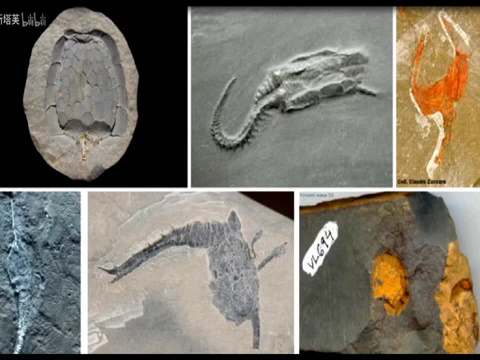 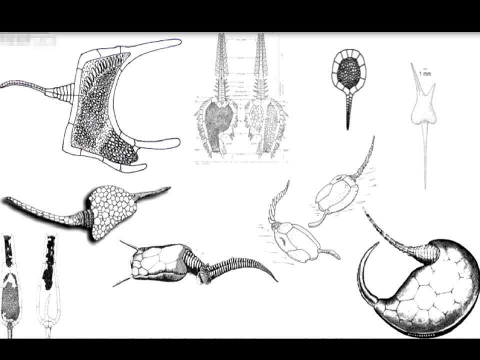 break all symmetry patterns and are simply a pile of geometric shapes randomly stacked together. Looking at these creatures which paleontologists have reconstructed, one would never guess that they are actually animals. Faced with such a bizarre looking creature, we can't even imagine. 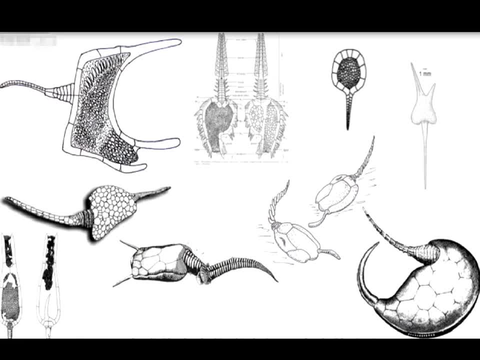 how food and water flow inside their body or how they evolved down such an unusual path. Many science fiction writers nowadays have poor imagination. They exhaust their creativity and come up with alien language. They are not sure what to do with their soul. They are not sure who to. be or what to do with their body. They are not sure what to do with their soul. They are not sure what to do with their body. They are not sure what to do with their soul. They are not sure what to do with their soul. 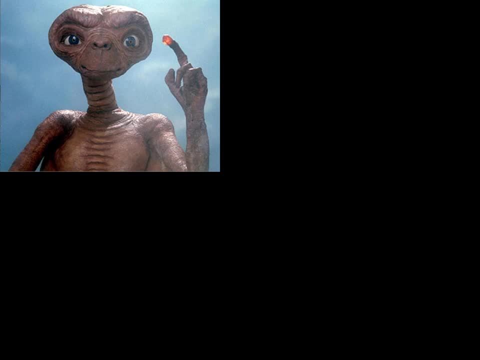 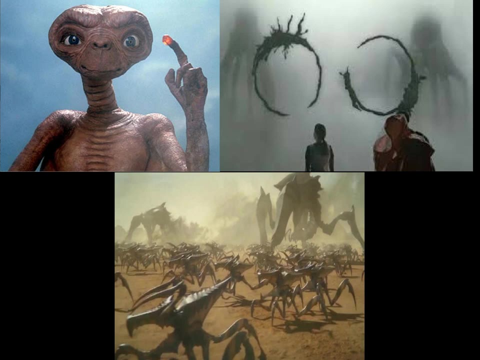 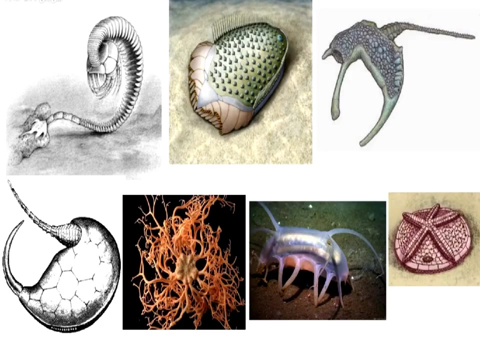 creatures that cannot escape the categories of vertebrates, arthropods and mollusks. However, on our planet there exists a group of animals that can easily exceed the limits of human imagination: Echinoderms. Whether extinct or extant, any one of them can subvert. 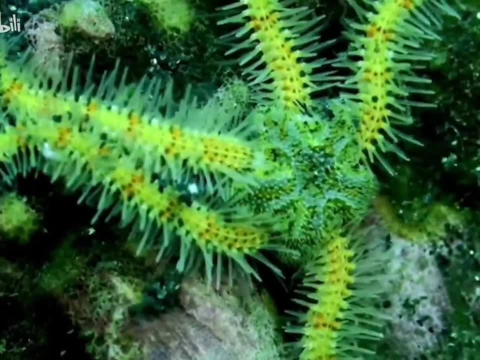 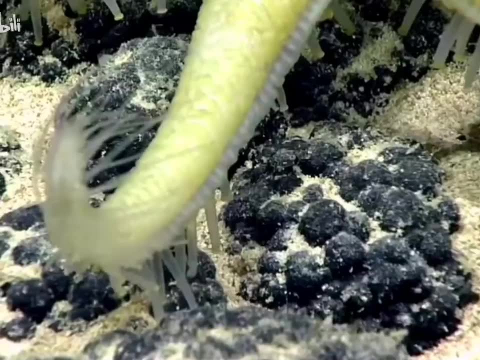 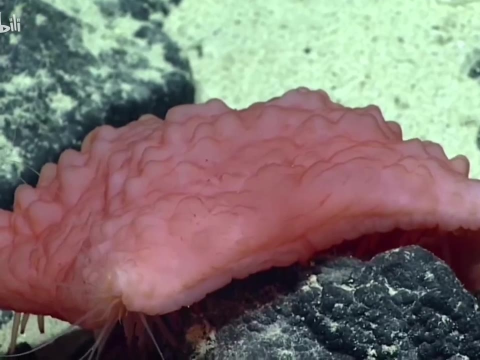 human imagination. Echinoderms are wild and free in their external appearance, but extremely conservative in certain aspects, such as never-evolving eyes, nervous systems or circulatory systems. From their names we can tell that Echinoderms have. 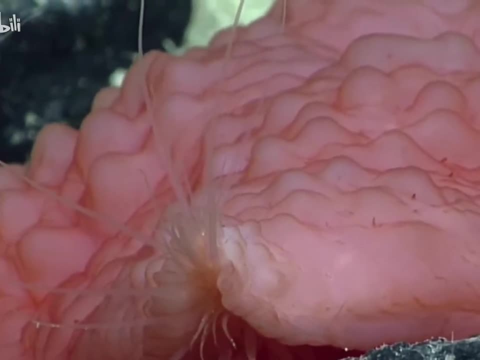 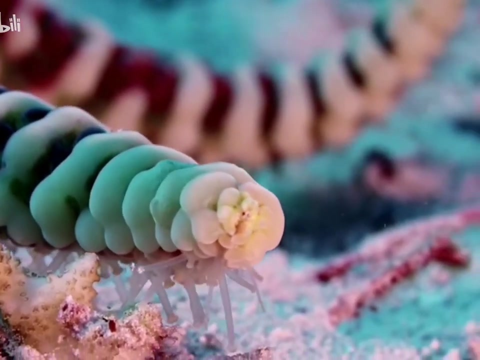 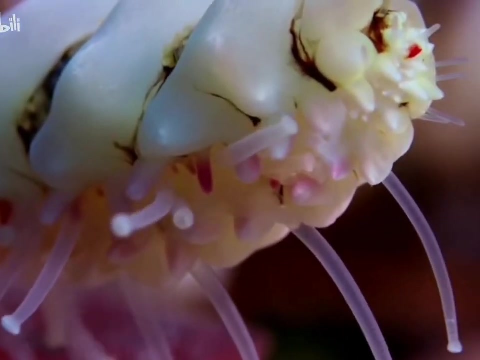 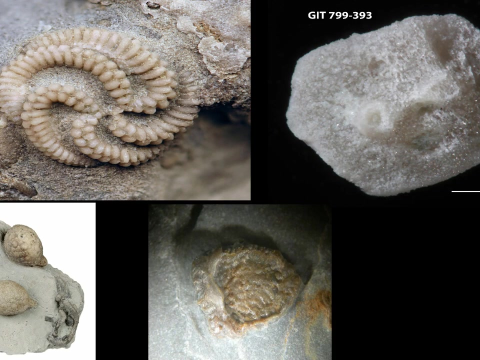 never left the ocean, let alone fresh water or land. This has cost them a great price in every major extinction event throughout history, causing the Echinoderm family to constantly shrink over the past 400 million years. Names like Edrioasteroids, Cyclocystodes, Cystodes, Camptostromates and Ophiocystodes. 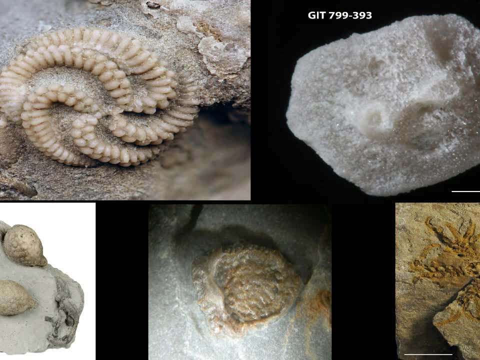 have become ancient mysteries buried in the rock layers. However, from another perspective, Echinoderms can always survive by relying on their endless creativity, using their odd species to twist and turn their bizarre bodies and bloom a variety of oddities on this planet. 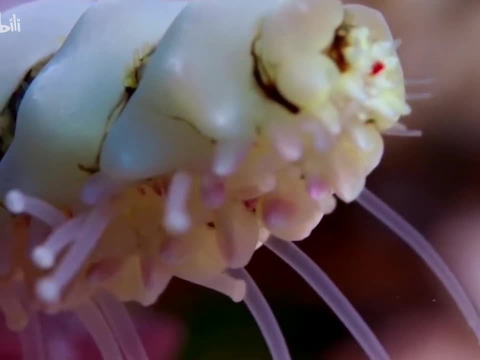 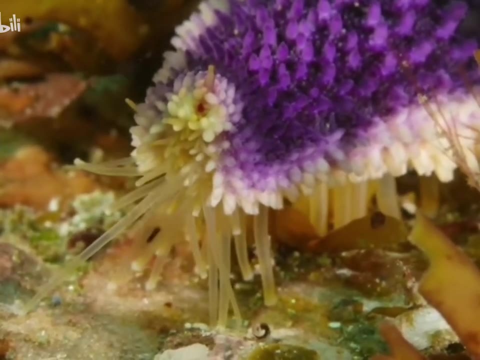 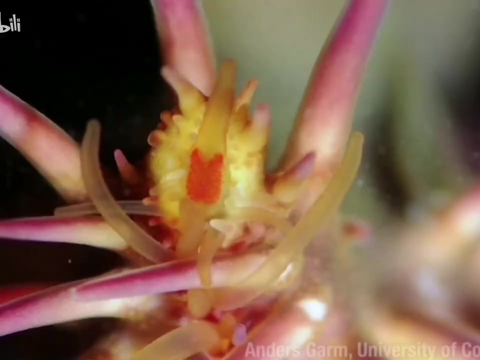 In my opinion, any group of animals that has gone through the process of evolution, no matter what path they have taken or whether they have succeeded or not, is a magnificent epic that can always make me feel amazed. Only when facing Echinoderms, my heart feels no emotion and I can only think of laughing. 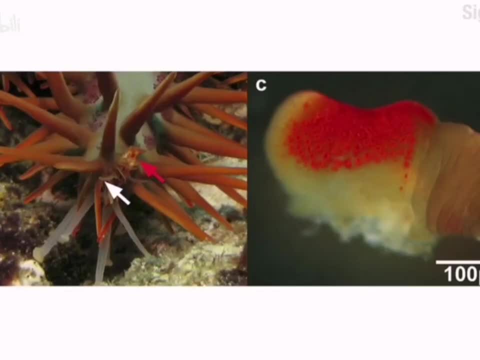 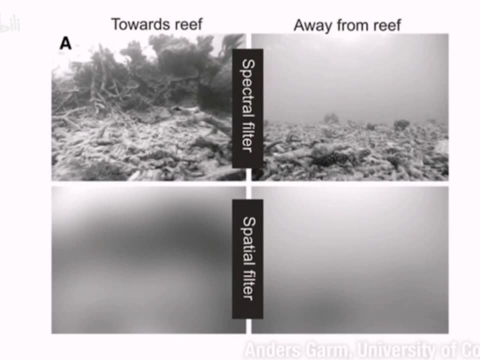 That's all for today's video. Thank you for watching and I hope you can subscribe to my channel. I'll share more interesting knowledge about prehistoric creatures. Goodbye.